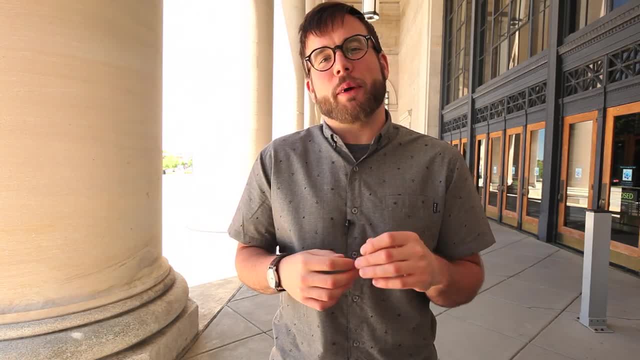 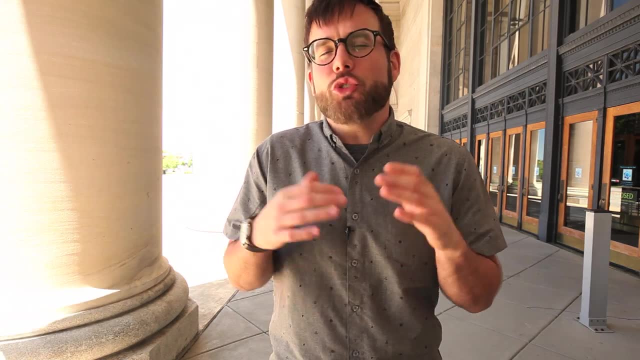 Hey everybody, I'm Dr Jeremy Hoffman, the Climate and Earth Science Specialist here at the Science Museum of Virginia. Today let's look into something you've probably heard about a lot recently: Just what is the scientific difference between weather and climate. 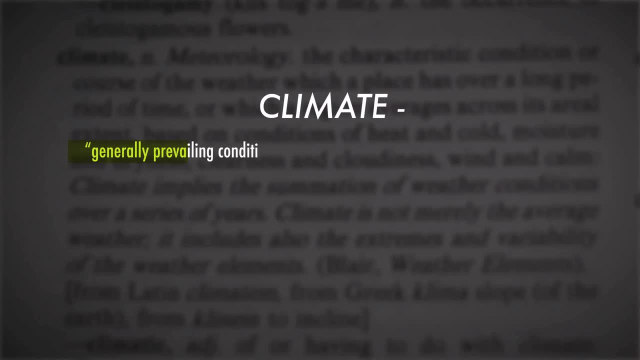 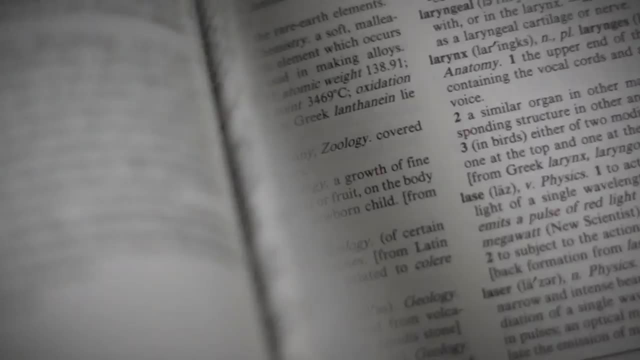 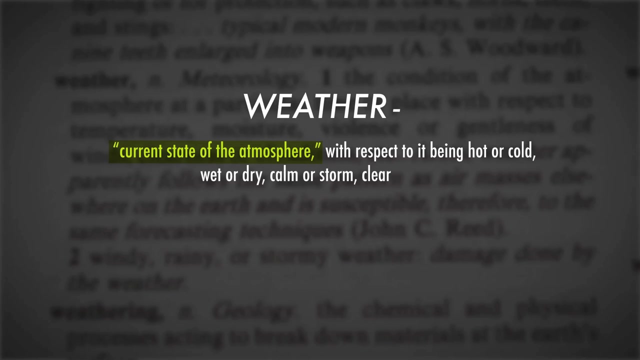 The dictionary defines climate as the generally prevailing conditions of a region, such as its yearly temperatures, winds and precipitation, averaged over a series of years, while the weather is defined as the current state of the atmosphere with respect to it being hot or cold, wet or dry, calm or storm, clear or cloudy. 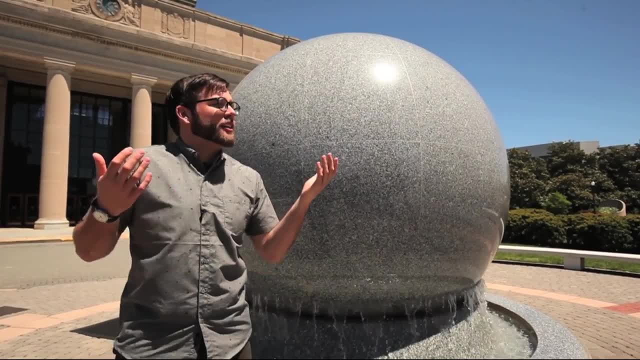 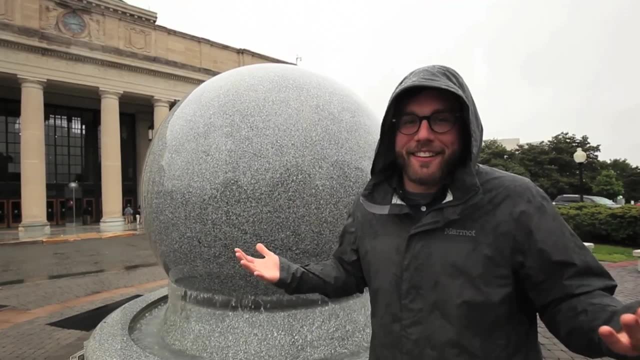 For example, the weather one day can be clear and sunny, with a light westerly wind, And the next day it can be cold and rainy with a chance of thunderstorms. But how can we get a better feel for what climate really is? 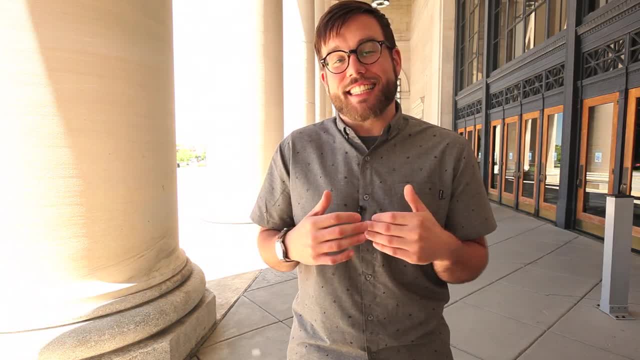 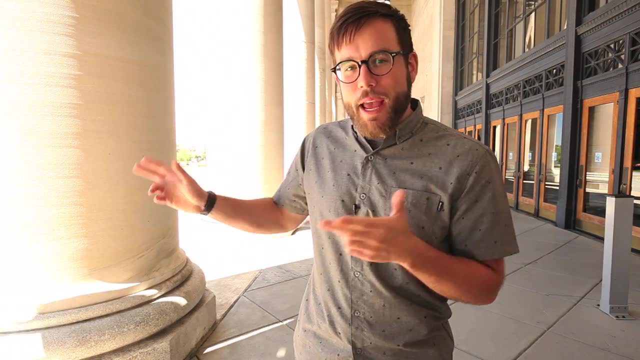 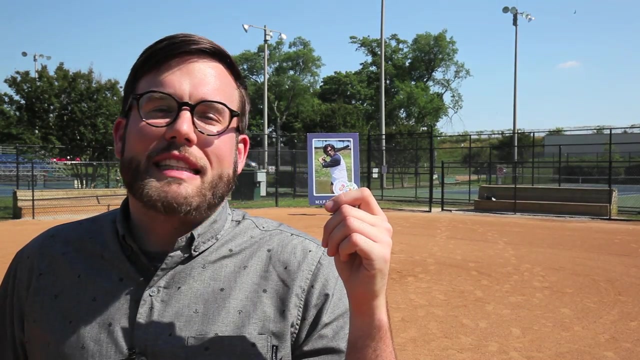 Let's take a look at a couple examples so that we can better recognize the differences between weather and climate. In order to do this, we have to go somewhere. you might not know, You might not expect To the baseball diamond- Consider Perbier's little-known baseball career. 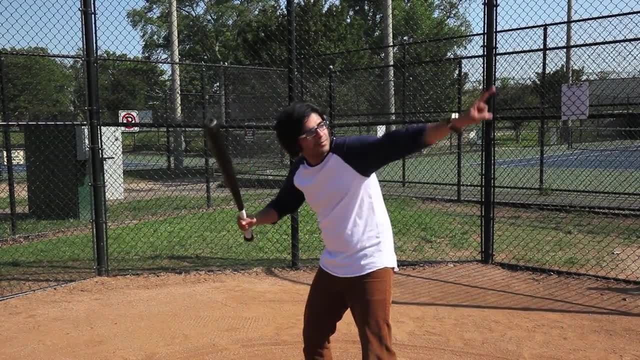 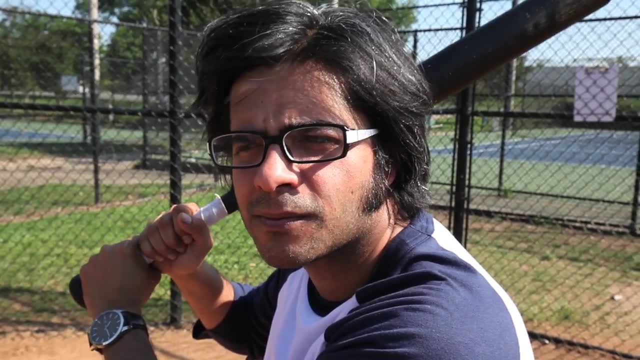 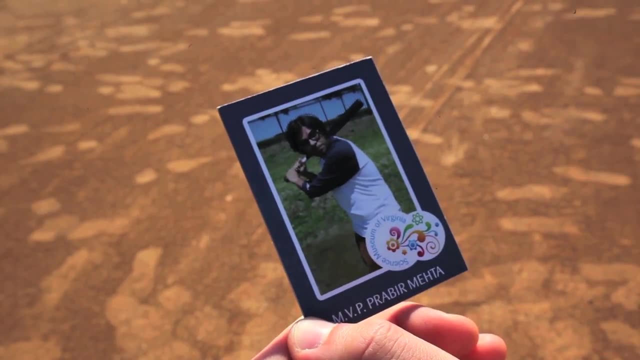 When Perbier goes up to bat, he can hit a home run, Or he can bunt. More than likely, though, he's going to strike out. Perbier's at-bat is like baseball weather- Perbier's baseball card, on the other hand. 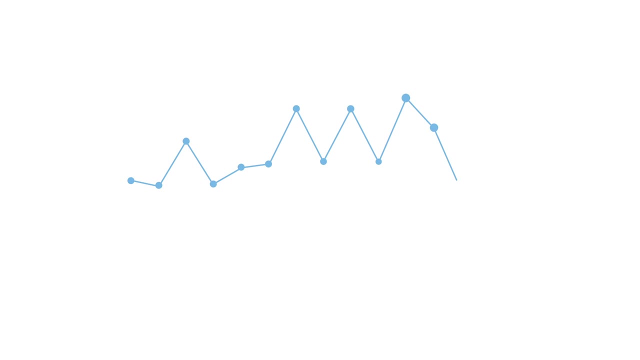 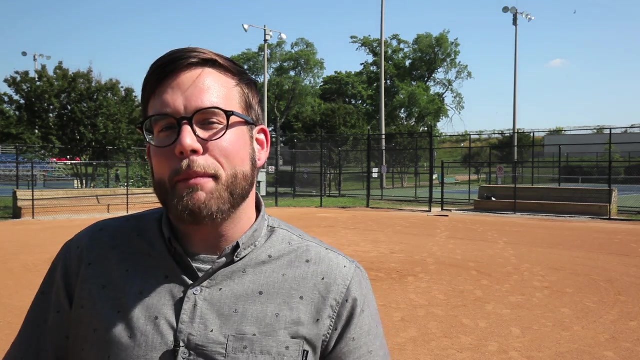 tells us about his long-term average chance of getting a hit, also known as his batting average. This is like baseball climate- the long-term average of at-bats, just like climate, is the long-term average of weather. But let's look at another way we can think about this science. 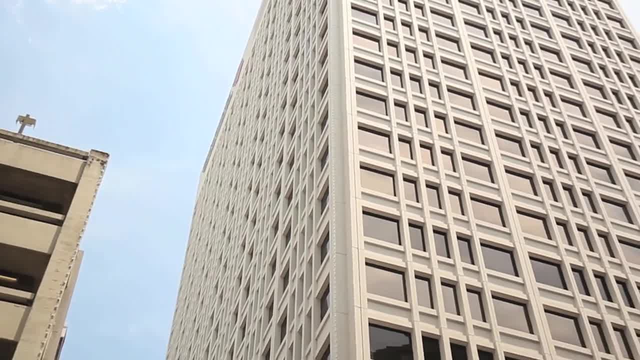 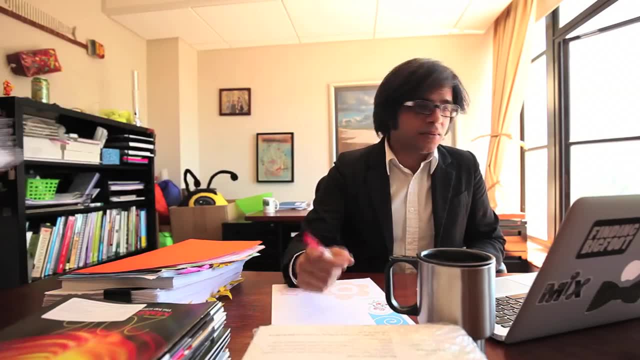 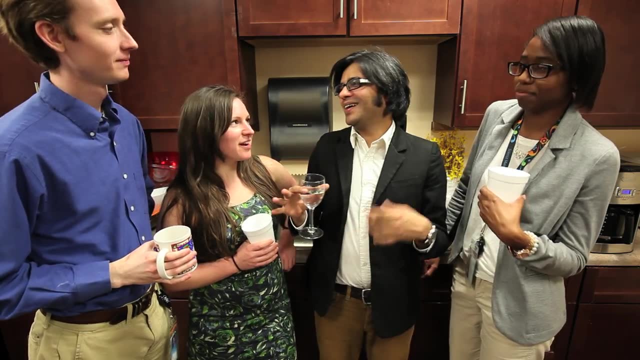 using human psychology. Perbier has had an especially rough day at work. He's stressed, he's busy, he's upset and he's quiet. But everyone knows Perbier to be a really outgoing and fun guy, And so I said I think it's the same difference.